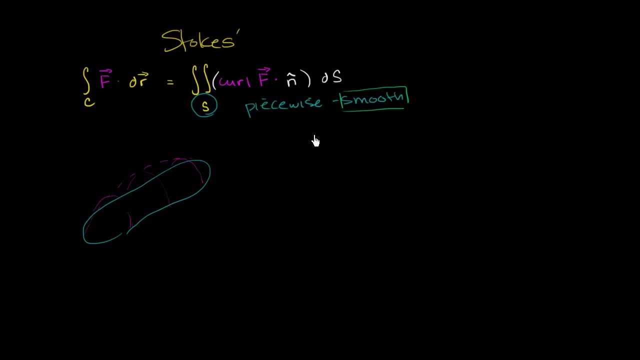 is that you have continuous derivatives And since we're talking about a surface, we're going to think about continuous partial derivatives, regardless of which direction you pick. So this is continuous derivatives, And another way to think about that conceptually is that if you pick a direction, 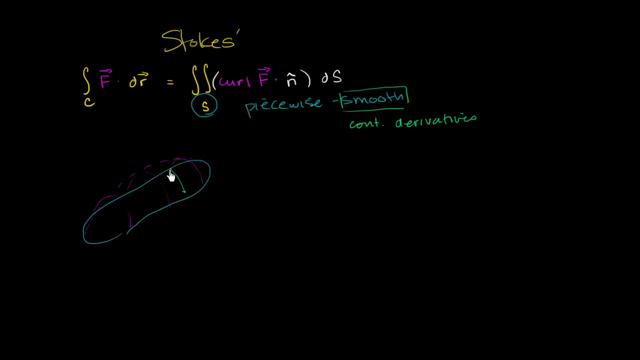 all the surfaces are continuous On the surface. if you say that we go in that direction, the slope in that direction changes gradually. It doesn't jump around. If you pick this direction right over here, the slope is changing gradually, So we have a continuous derivative. 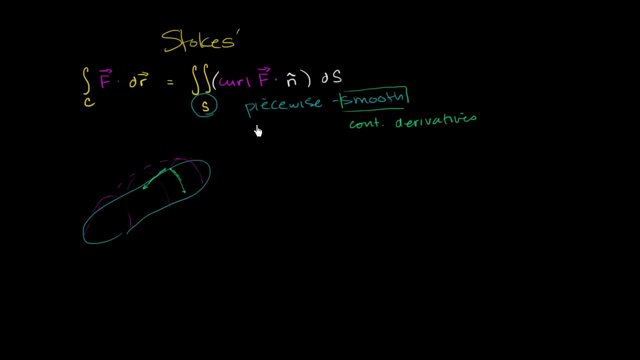 Now you're like: well, what does the piecewise mean? Well, the piecewise actually allows us to use Stokes' theorem with more surfaces, Because if we have a surface that looks like, let's say, a surface that looks like this, Let's say, it looks like a cup. 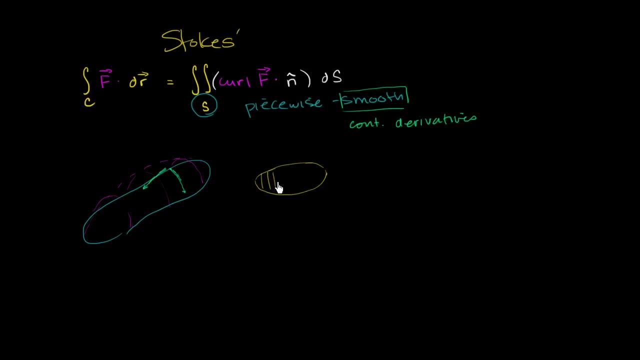 So this is the opening of the top of the cup. Let's say it has no opening on top, so we can see the back side. This is the back side of the cup And this is the side of the cup. And then this right over here is the bottom of the cup. 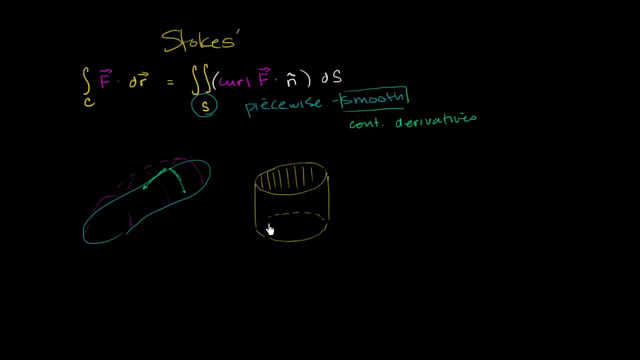 And if it was transparent we could actually see through it. So a surface like this is not entirely smooth, because it has edges. There are points right over here. So this edge right over here, if we pick this, let's say we pick this direction to go. 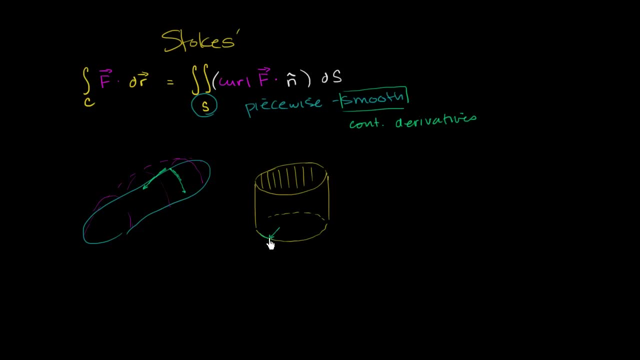 And if we go in this direction, along the bottom, then right when we get to the edge, then all of a sudden the slope changes dramatically, It jumps. So the slope is not continuous at that edge, The slope jumps, And then we start going straight up. 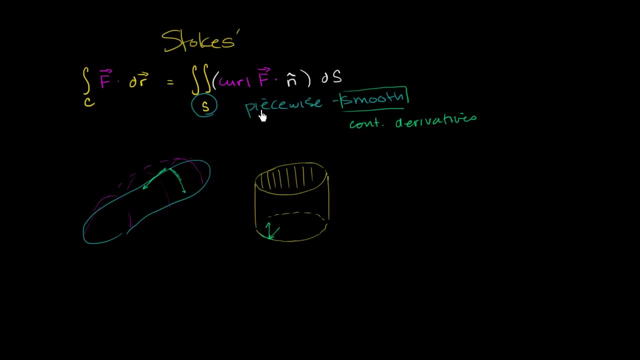 And so this entire surface is not smooth, But the piecewise actually gives us an out. This tells us that it's okay as long as we can break the surface up into pieces that are smooth, And so this cup, we can break it up. 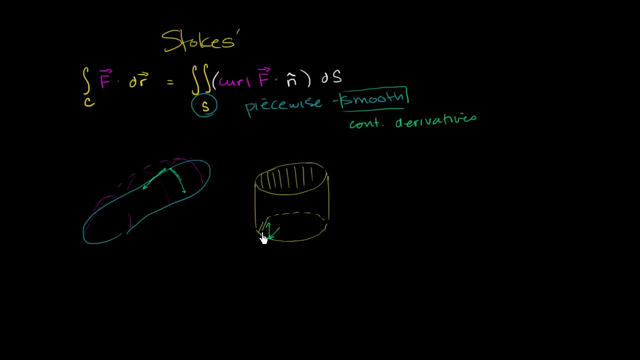 And we've been doing this when we've been tackling surface integrals. We can break it up into the bottom part, which is a smooth surface- It has a continuous derivative- And the sides, the sides, the side which kind of wraps around. 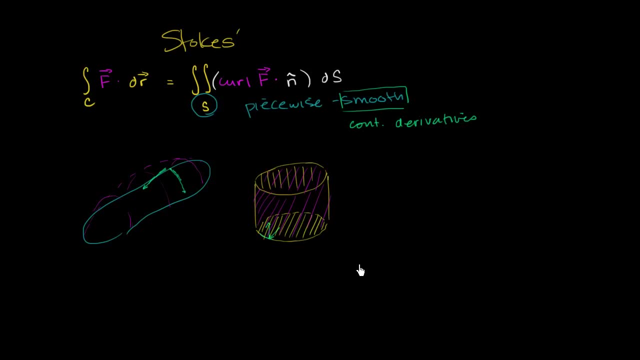 is also is also a smooth surface. So most things that you will encounter in a traditional calculus course actually do, especially surfaces, do fit piecewise smooth And the things that don't actually are fairly hard to visualize, And I imagine these ultra pointy 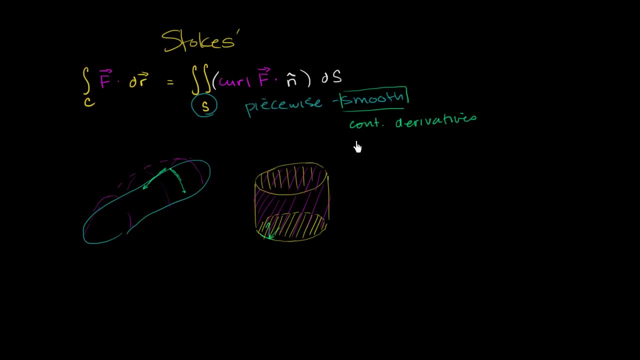 fractally looking things, where it's hard to break it up into pieces that are actually smooth. That's for the surface part, But we also have to care about the boundary in order to apply Stokes' theorem. And that's that right over there. 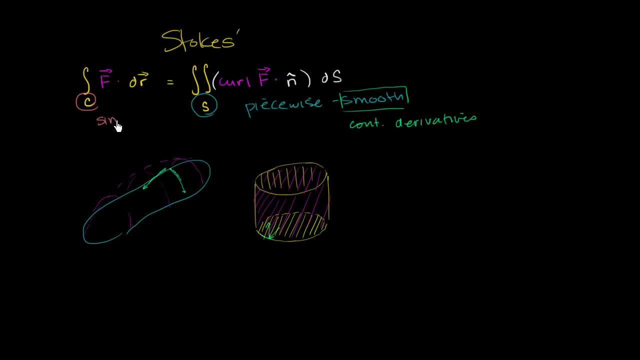 The boundary needs to be a simple, which means it doesn't cross itself, a simple, closed, piecewise, smooth boundary. So once again, simple and closed, that just means so this is not a simple boundary if it's really crossing itself, if it intersects itself. 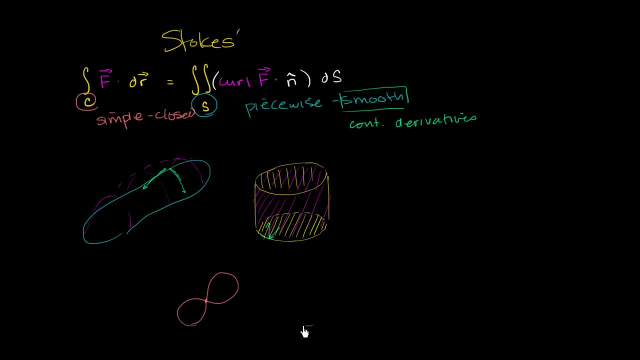 Although you could break it up into two simple boundaries, But something like this is a simple boundary, So that's a simple boundary. right over there, It also has to be closed, which really means it just loops in on itself. You just won't have something like that. 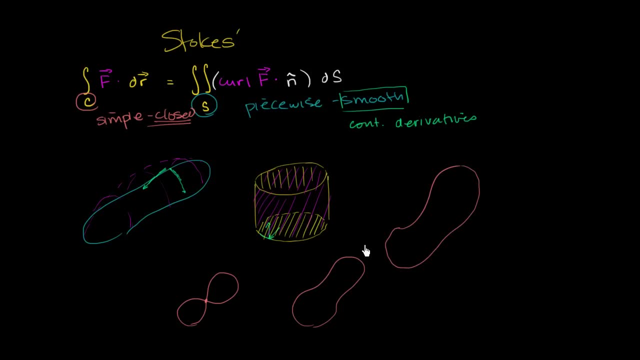 It actually has to close, It actually has to loop in on itself, in order to use Stokes' theorem, And once again, it has to be piecewise smooth. But now we're talking about a path or a line or a curve, like this: 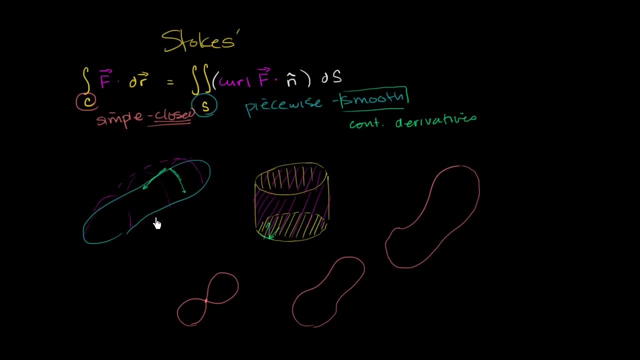 And piecewise smooth just means that you can break it up into sections where the derivative is continuous. The way I've drawn this one, this one and this one, the slope is changing gradually. So over there the slope is like that It's changing gradually. 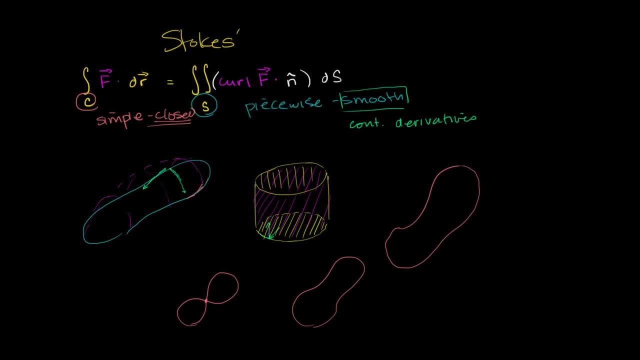 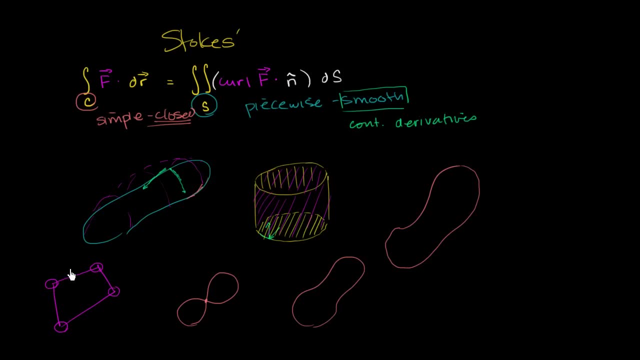 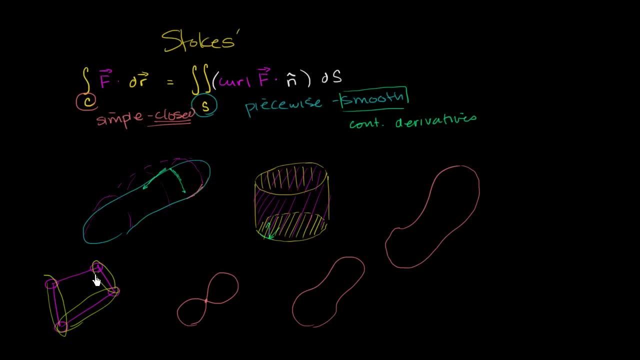 That line right over there is smooth, That line is smooth And that line is smooth. And we've done that. When we've evaluated line integrals, We've broken them up into smooth segments that we can then use to actually compute the line integral. 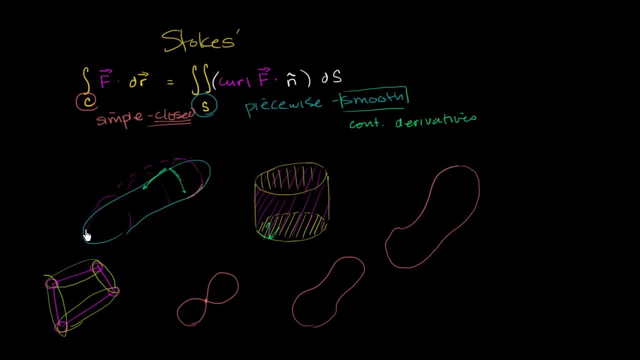 So if you find, if you have a boundary where the, or if you have a surface that is piecewise smooth and its boundary is a simple, closed, piecewise smooth boundary, you're good to go.